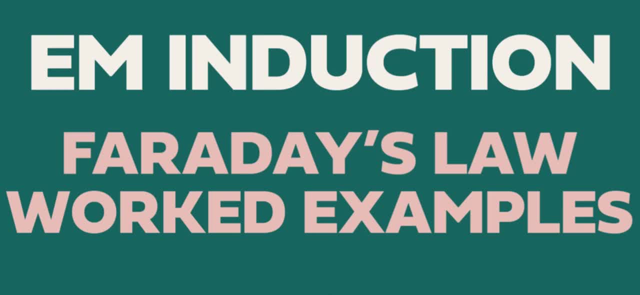 In this video I'll be discussing two worked examples on Faraday's Law. This video is part of a playlist of videos on electromagnetic induction and directly follows the previous video in which we discussed Faraday's Law. To follow this video and get the most out of it. 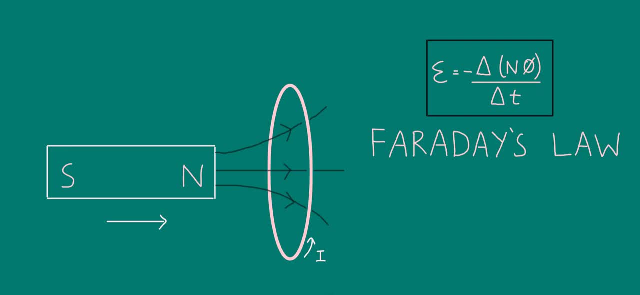 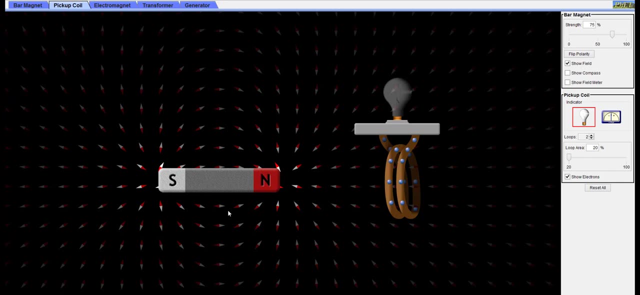 you need to have some familiarity with Faraday's Law, So if you don't, I recommend you check out the previous video. first, Let's take a look at the first worked example. In the previous video we explored the various factors that determine the induced EMF that develops. 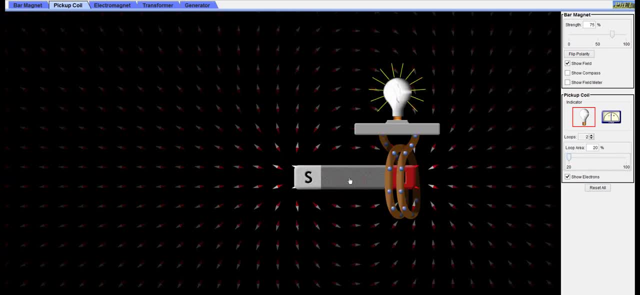 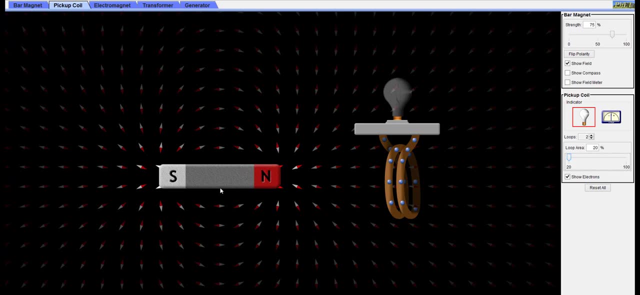 when a magnet is moved towards a coil of wire, For example, increasing the speed at which the magnet is moved leads to a greater induced EMF. One thing we didn't look at is what happens if we push the magnet right through the coil. So let's do that. 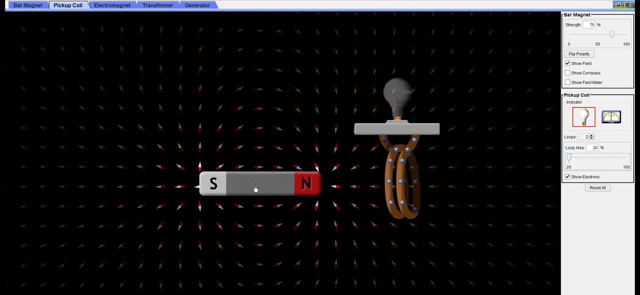 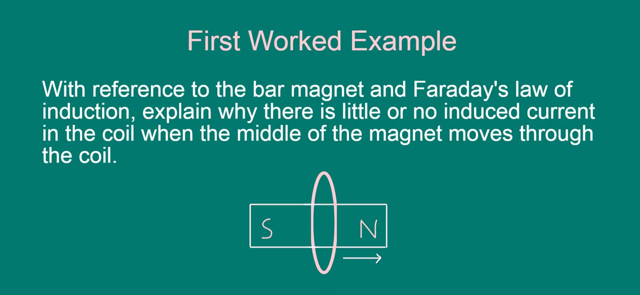 Notice anything interesting. For some reason, when the middle of the magnet moves through the coil, the current stops flowing and the lamp stops glowing. This is the first puzzle we want to solve. So our first worked example is with reference to the bar magnet and Faraday's Law. 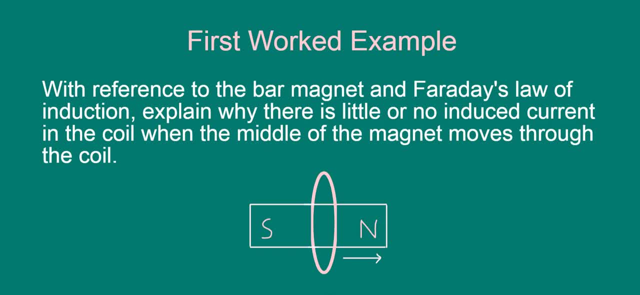 of Induction. explain why there is little or no induced current in the coil when the middle of the magnet moves through the coil? Why not pause the video and see if you can figure this out for yourself? When you're done, I'll be happy to answer your questions Until next time. bye for now. 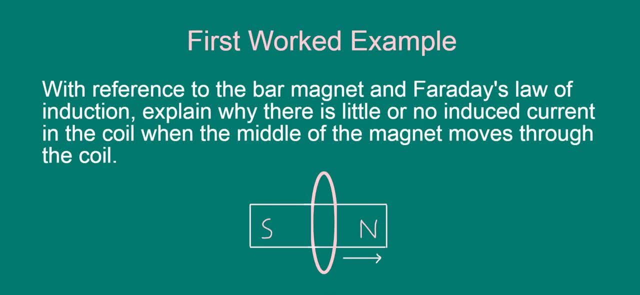 Okay, welcome back. So we know that the magnetic field lines outside a bar magnet are directed from north to south and are non-uniform. Inside the magnet, however, the field lines are directed from south to north and are basically uniform as shown. So the field 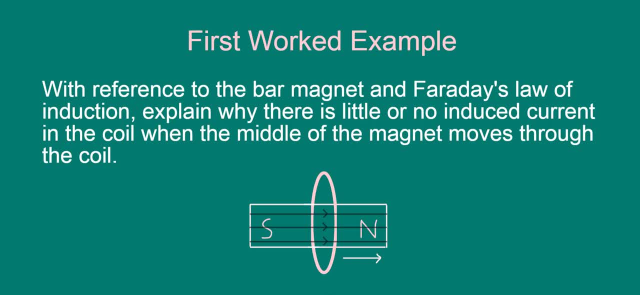 lines are shown in black. So when the middle of the magnet passes through the coil during a time interval- delta t- the magnetic field lines are directed from north to south and are non-uniform. There's virtually no change in the magnetic flux density at the coil. 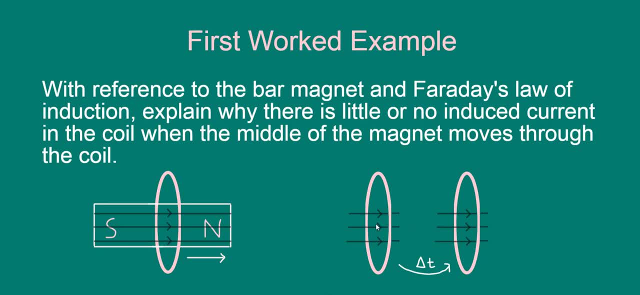 What this little sketch here is showing is the magnet being pushed through over a little time interval, delta t. I haven't actually drawn the magnet for clarity, but what you can see is the magnetic field lines right which correspond to the magnetic field line in the interior or the 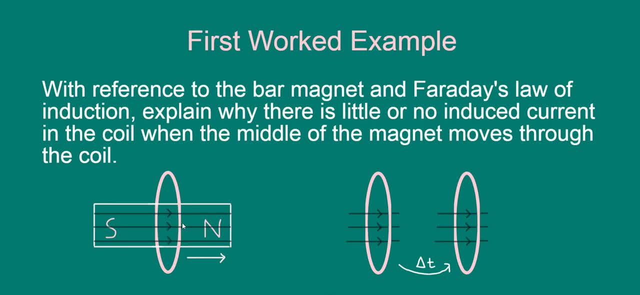 middle of the magnet And, as I mentioned, because it's effectively a uniform field as the magnet pushes through the coil, there's virtually no change in the magnetic field or magnetic flux density in the coil over this period of time- delta t. So what this means is that there is no 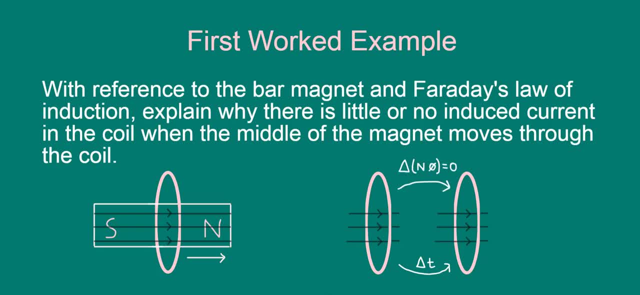 change in the flux linkage. Remember that flux linkage is given by the product of n, the number of turns of wire, times phi, the magnetic flux for an aerial coil, And n is constant. There's no change to that, of course, And phi there used to be several times and there's several times. И. which you'll notice is that the fluxastics use second method. So delta p, where it's a number of turns of wire times P, which is equal to E. The magnetic flow fabric is a州 yłye rank of んな D, where it's δ. So what this means is that there is no change in the flux linkage. Remember that flux. 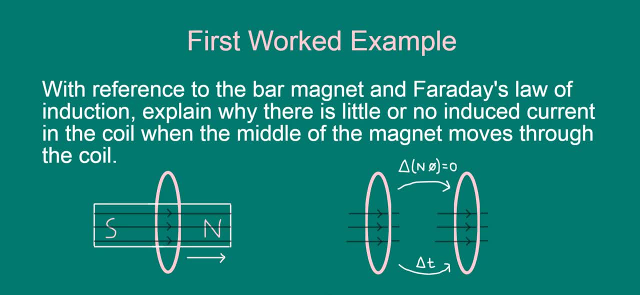 There's no change to that. of course, And phi, the flux is also constant because the flux density isn't changing, B isn't changing and the area through which it acts or passes through A is also unchanging. So there's no change in flux linkage here. 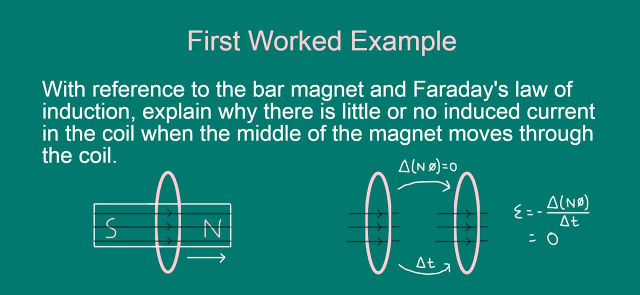 And so from Faraday's law, which states that the induced EMF is given by the negative rate of change of flux linkage, we can see that the induced EMF must be zero if there is no change in flux linkage, And this is what explains why there's little or no induced current in the coil. 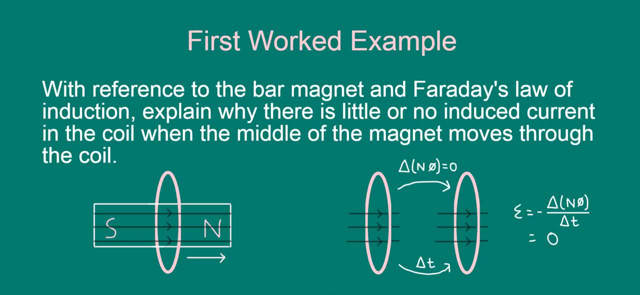 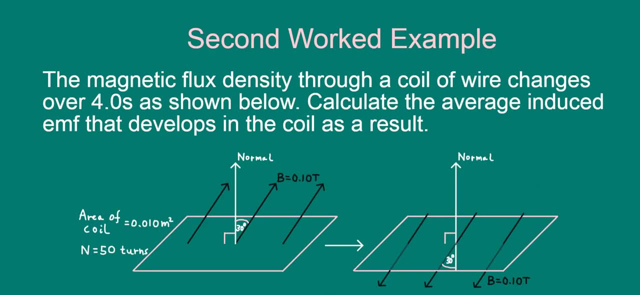 when the middle of the magnet passes through the coil. Let's now take a look at our second worked example. The magnetic flux density through a coil of wire changes over 4.0 seconds, as shown below. Calculate the average induced EMF that develops in the coil as a result. 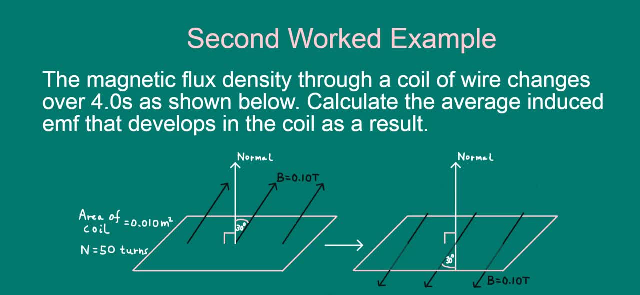 So once again we've got a coil of wire, but this time it's rectangular or square-shaped, as shown here. We're told the area of the coil of wire: 0.010 meters squared. You're also told the number of turns of wire in the coil: it's 50 turns. 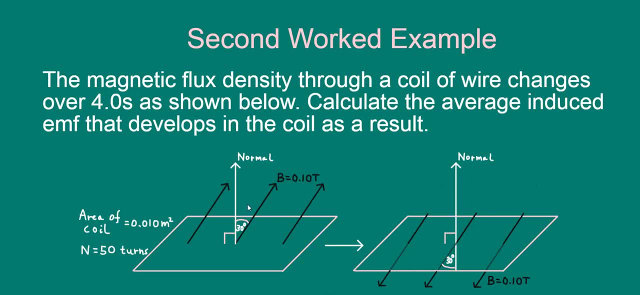 And you can see there's a magnetic field. you can see these magnetic field lines poking through this area shown in black And we're told the flux density, the magnitude of the flux density: 0.10 tesla. And what happens is that over the course of 4 seconds, this flux density changes, changes direction, as you can see. 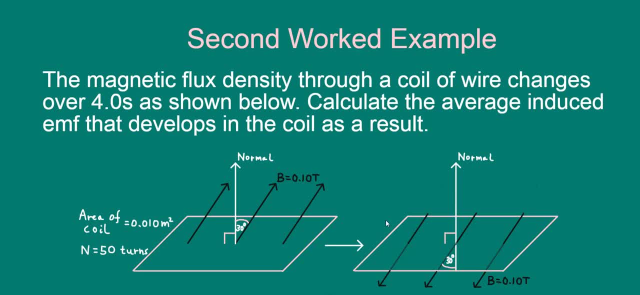 Right, so there's no change to the magnitude of the flux density, but obviously a big change in direction. And note here these angles are 30 degrees here and here as well. So once again, I encourage you to pause the video and see if you can answer this yourself. 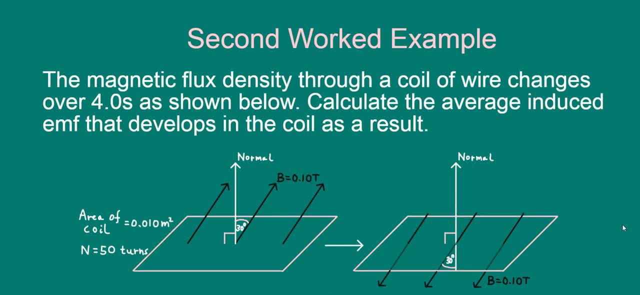 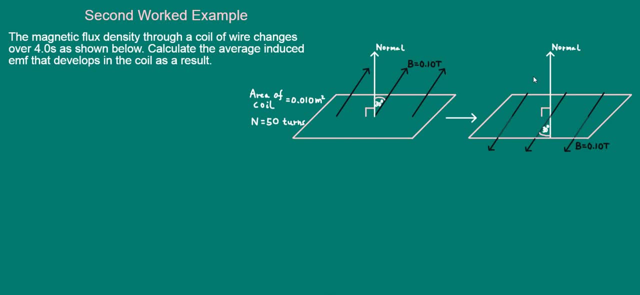 And once you've had a go at that, unpause the video and we'll go through it. Okay, welcome back. So to figure out the induced EMF, we're going to have to, of course, work out how the flux linkage changes. 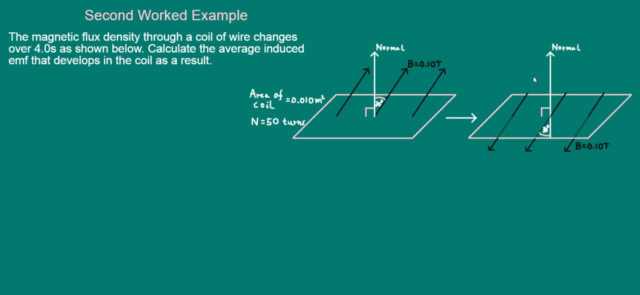 Over the course of 4 seconds. So we need to work out the initial flux linkage And to do that, of course, we need to work out n times. the initial flux, which is represented by phi t equals 0.. And this initial flux is just given by the component of the flux density parallel to the normal. 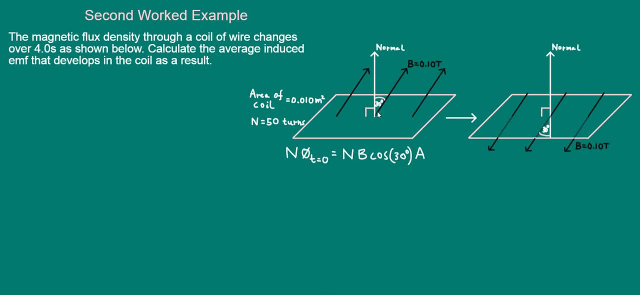 And so that's given by b cosine 30, multiplied by the area of the component, And this is the angle that we're going to have to work out through which the field lines are poking through. Now we also need to figure out the flux linkage through the coil: 4.0 seconds later. 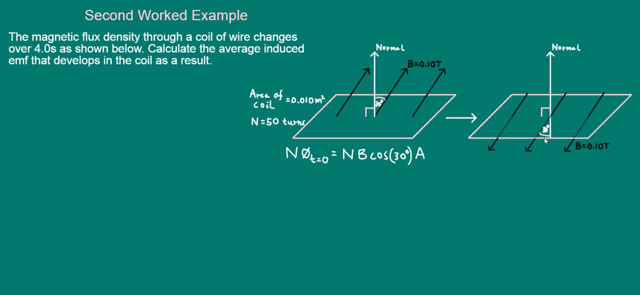 And essentially it's the same procedure, except we need to be a little bit careful about the angle we have to use. The angle we have to use now is 30 degrees plus 180 degrees here. Okay, so that's the angle that the field lines or the flux density makes with the normal. now 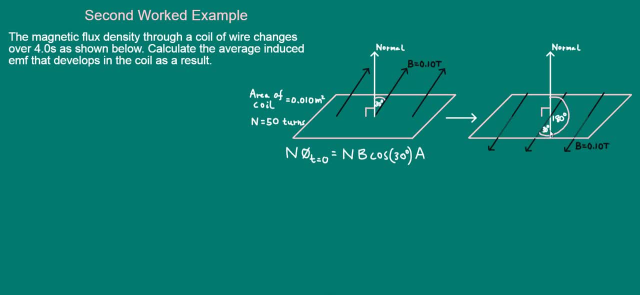 It's now 210.. It's sort of like the angle of interest is the angle between the direction in which the field lines are pointing and the direction in which the normal is pointing. So once we've established that the flux linkage through the coil then is just n times b times cosine, 210 degrees times a. 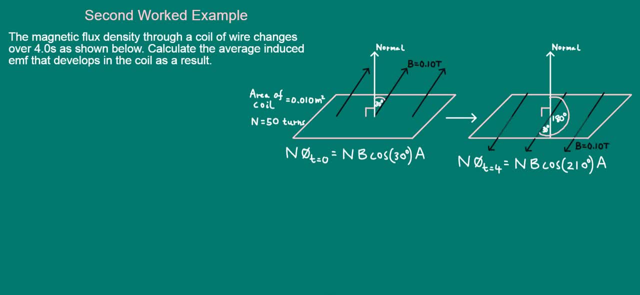 Now, once we have these two things figured out, we can, of course, work out the change in flux linkage, which is just the flux linkage at 4 seconds minus the flux linkage at the start, And if you take out a common factor of nba, we can get this expression here: 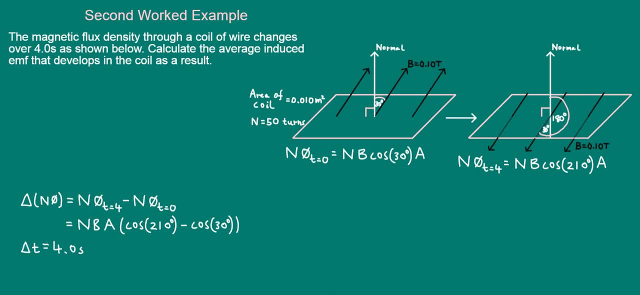 And we know that the change takes place over 4.0 seconds. So if we put all of this together we can work out the induced EMF that develops via Faraday's law. So if you just plug in all the numbers here and you work out the change in flux linkage divided by the time,